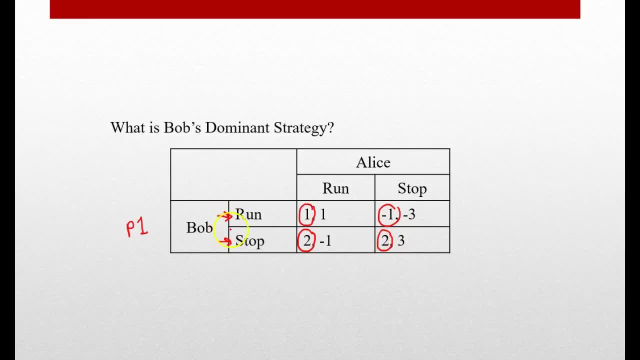 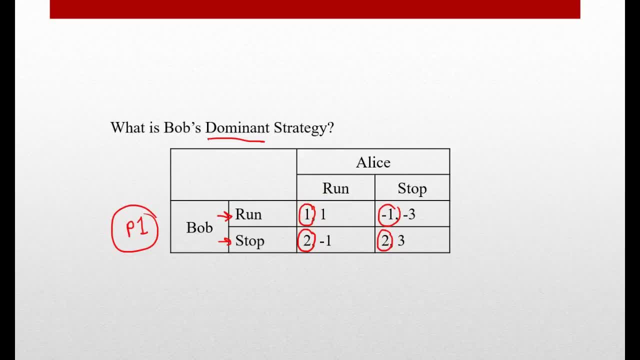 look and check out. Let's keep Alice's strategy the same each time. So let's look and see what happens if Alice chooses to run. What should Bob choose? Okay, so if Alice chooses to run, what should Bob choose? Should he choose to run or should he choose to stop? Now remember: the higher the number, the better the payoff. So we have one and two. Well, it appears that we should choose to stop. Okay, so in this first instance, 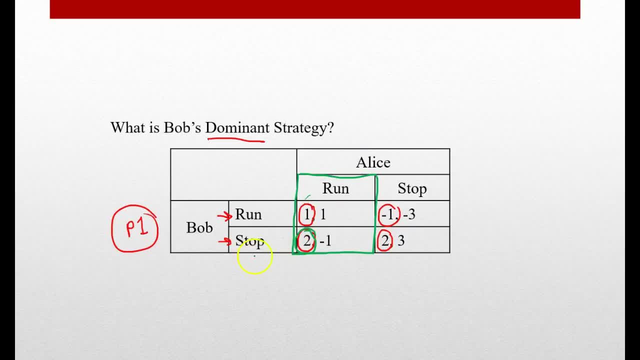 if Alice chooses to run, we should choose to stop. Bob's best interest is to stop. Now. let's go over to the stop column. Okay, here we are. What if Alice chooses to stop? What should Bob choose? Well, we have negative one and we have two. What's the better payoff? Well, positive is always better than negative, right? So two is a higher, So Bob should choose to stop Now. in either case, whatever Alice chooses, what should Bob choose? Well, Bob should choose to stop. 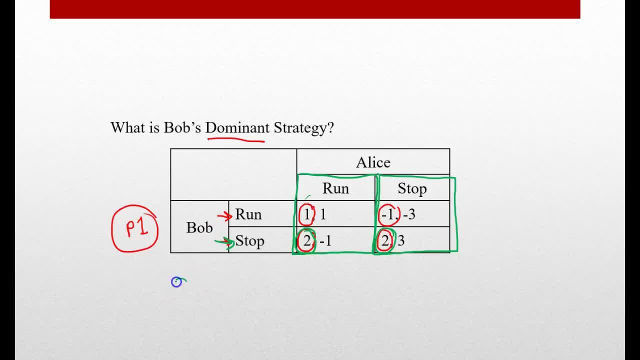 Bob should choose to stop. So what that means is stop is going to be Bob's dominant strategy, Dominant strategy. So the cool thing about this is, if you ever figure out what your dominant strategy should be, you can always go with that And it's always going to be your best choice. You don't even have to think about the moves or try to analyze what the other player is going to do. 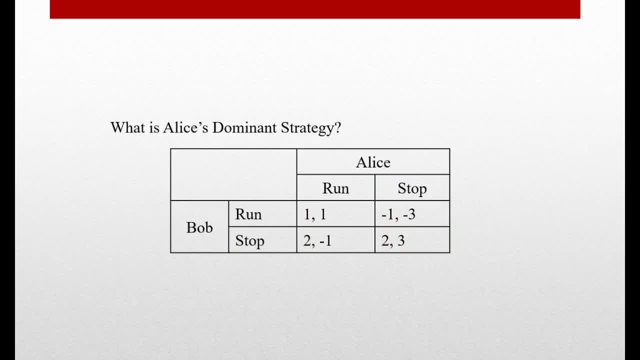 Right, No need for poker glasses here, Sunglasses. Now let's look at another example, But this time we want to figure out Alice's dominant strategy. So remember, in this case, Alice is going to be player two, since she's on top. here And again, she has two choices: She could either run or stop. Remember Alice, since she's player two, she's going to have columns Now, since she's also player two, that means the second number. 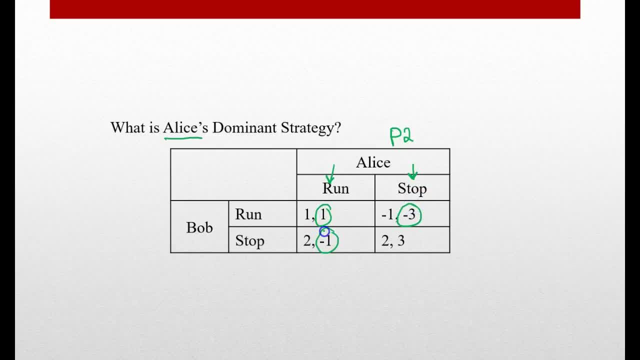 Player two, second number: Ooh, connections there. Okay, Means that all the second numbers are going to be her payoffs. So we can basically ignore Bob's payoffs, which are the first numbers right now. Okay, So we're trying to decide: should Alice run or should she stop. Now we're going to do the same thing we did before, but this time we're going to keep Bob's choices the same. So if Bob chooses to run, what is Alice's best decision? 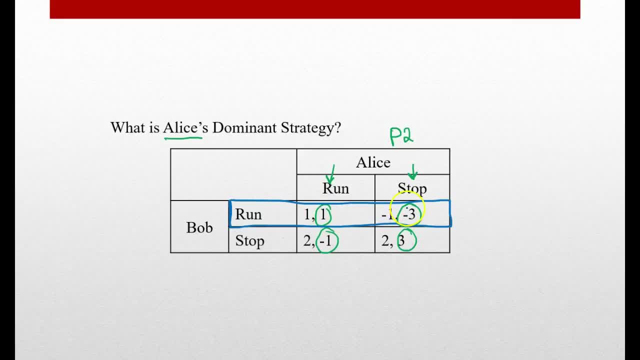 So if Bob chooses to run, should she choose to also run or stop? Well, one and negative three. I'm going to choose a positive number, right, Always a better payoff. So, Alice, the best choice would be to run. Okay, Now let's skip over to if Bob chooses to stop, what should we choose? Should we choose to run or stop? Well, negative, one or three. 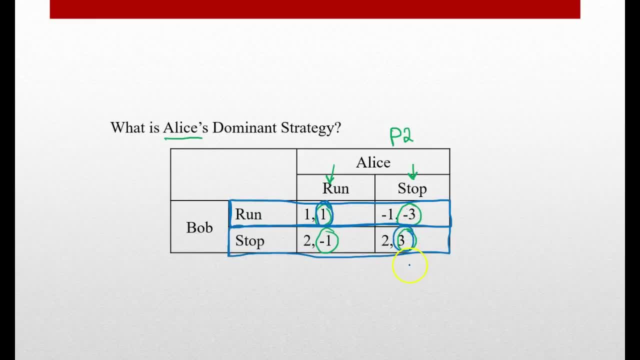 I'm going to go ahead with three, because that seems like a better option for me. Now there's a problem. Okay, If we look at this, if Bob chooses to run, Alice should also choose to run. right, That's what we said. But if Bob chooses to stop, Alice should choose to stop. So, depending on what Bob does, Alice should do something different. 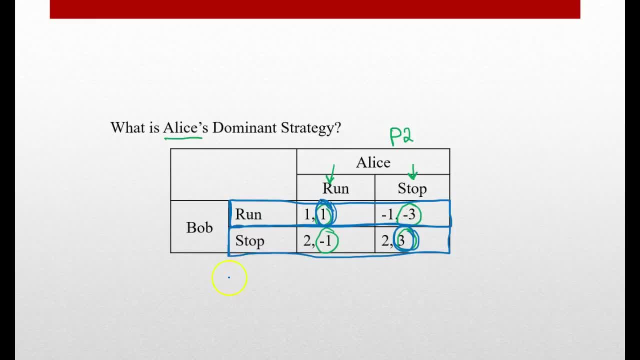 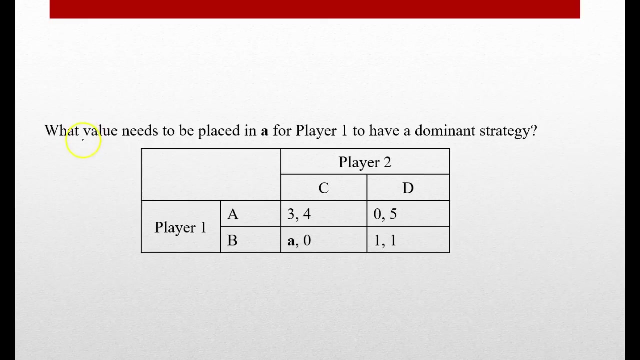 So since Alice doesn't have one strategy, that's always going to work. we would say: Alice does not have a dominant strategy, So no dominant strategy. So that's what we're going to go with here. So let's finish that up. Strategy- Okay, Now we have one more example we want to get through. So the last example is what value needs to be placed in A for player one to have a dominant strategy. So now we have a very general 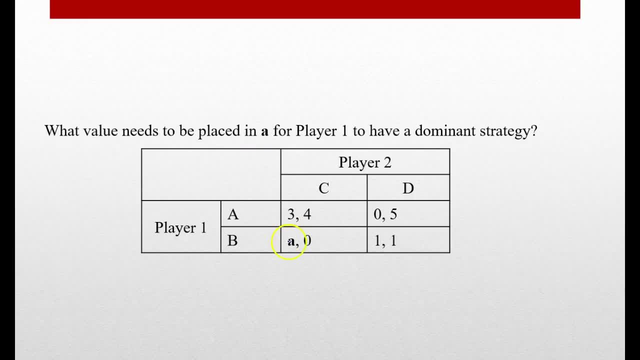 game matrix. Okay, And we're missing a number that we need to plug in for this little A, Lowercase A. So let's talk about this. So we have our player one over here, We have our player two. Notice that for player one, it has either the choice, the strategy of A or the strategy of B. So this was kind of like the run or. 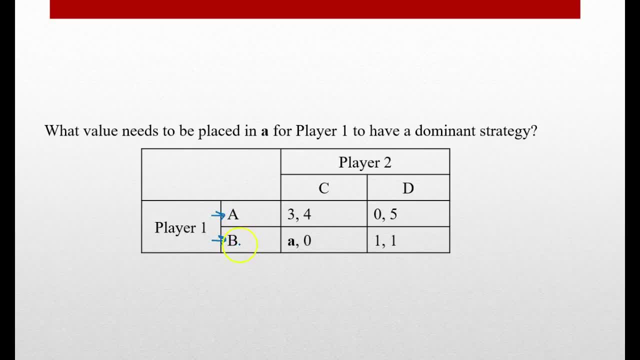 walk option or runner stay. Yep, that's what it was: Runner stay. And player two has the choices of C or D as their strategy. So just keep in mind these just represent different strategies. Don't get hung up on the fact that they're variables. So run, walk, stay, cooperate whatever it is. 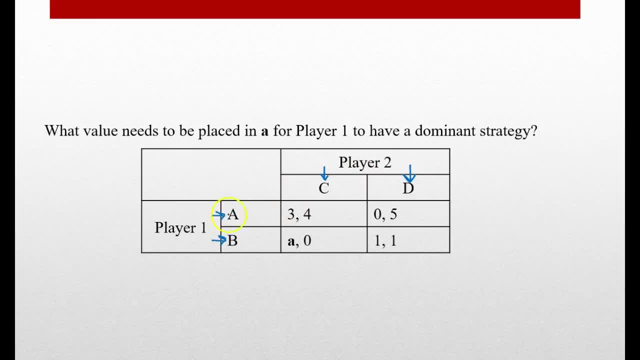 your strategy is Okay. now we want to figure out what player one's dominant strategy is. So player one, let's go ahead and just circle player one's payoff, so we can just concentrate on those and ignore player twos, because they don't matter when we're trying to find player one's dominant. 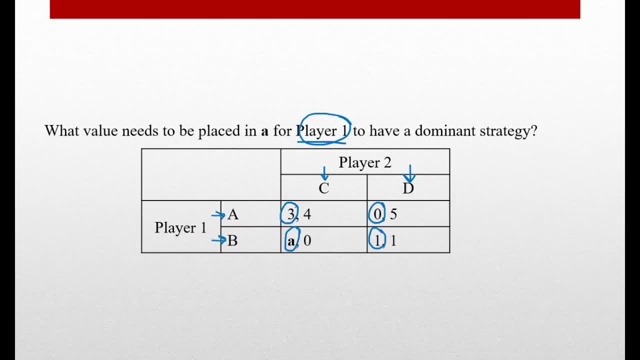 strategy. Okay, now remember, player one's dominant strategy depends on what player two chooses. So if player two chooses to go with strategy C, okay, we want to look at the payoffs for player one. So we have three and we have A, So we don't know which one should be bigger, right? 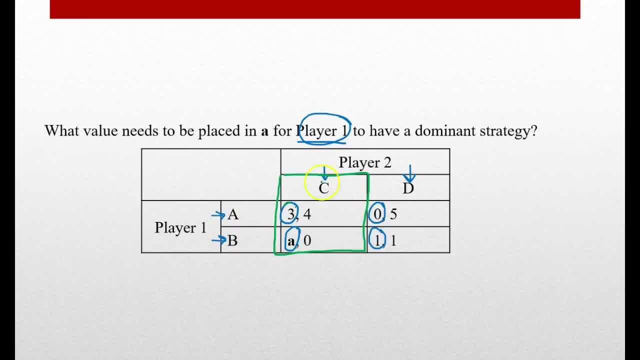 now We don't know the dominant strategy of player one, So let's put that on hold and come back to. if player two chooses C, Let's instead go to player two's choice of D. Okay, now, if we look here, you have: 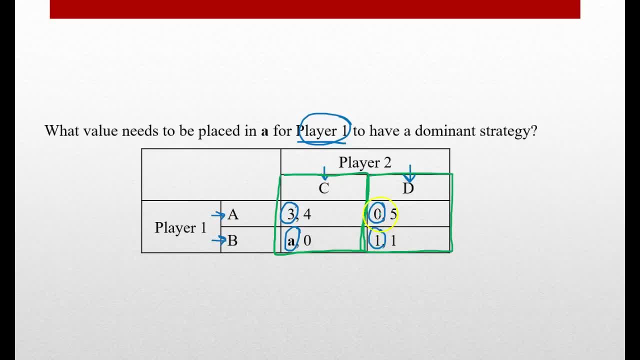 zero and one. Which one would be dominant? Which one would be a dominant strategy? Well, one would be the dominant strategy because it's higher right, So that one means player one should choose option B or strategy B. So if we come back to this first column, okay, where player two is choosing option C, you have